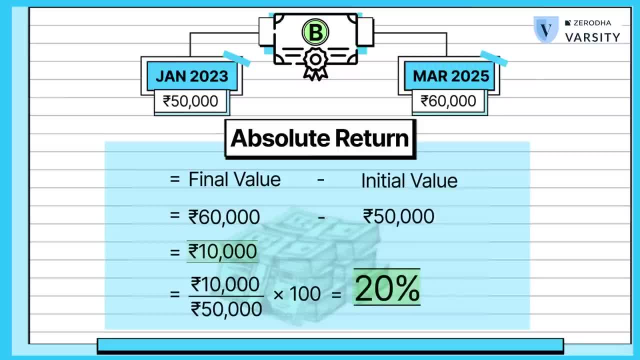 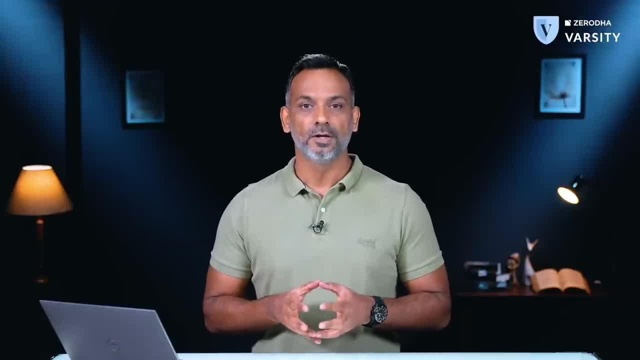 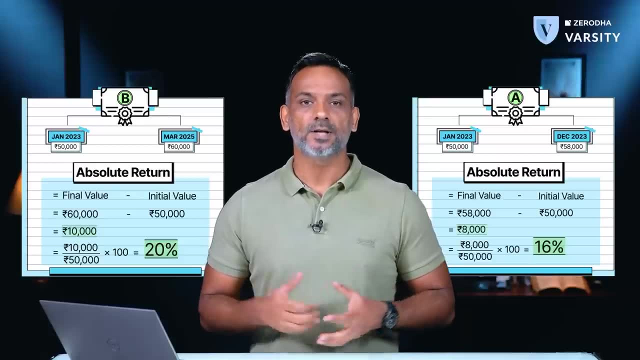 value, multiply by 100, and you get the value. So, if you do all this math, you will get the absolute return as 20%. Now, if you were to pick an investment, which stock would you choose? Would it be stock A or stock B? Well, this is a no-brainer Based on absolute return. 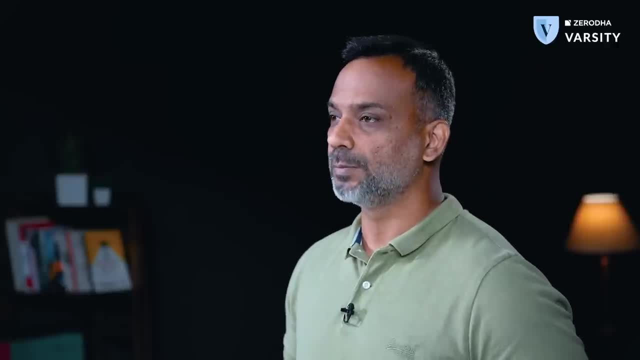 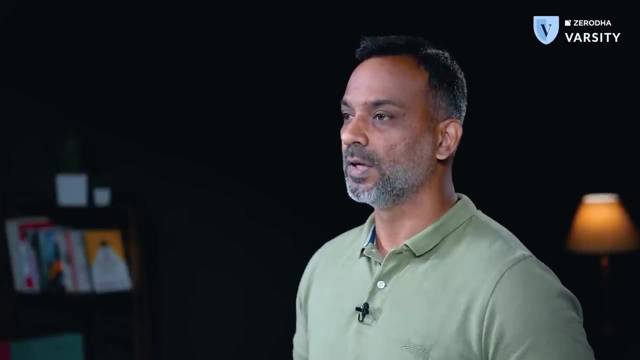 you would naturally pick stock B, But this is not the right approach. Whenever there is passage of time, you always have to consider time and the return over time. This is where the second metric comes into play, which is called the Compounded Annual Growth Rate, or CAGR. 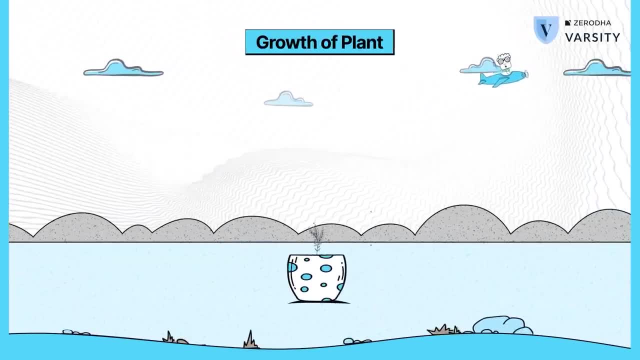 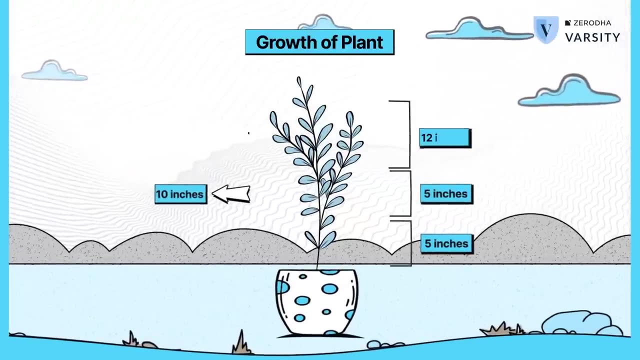 To put this in perspective, assume you get a 5-inch sapling from a nursery and plant that in your house. In the first year the plant grows to 10 inches. second year it grows to 22 inches and in the third year it grows to 45 inches. Here the absolute growth is: 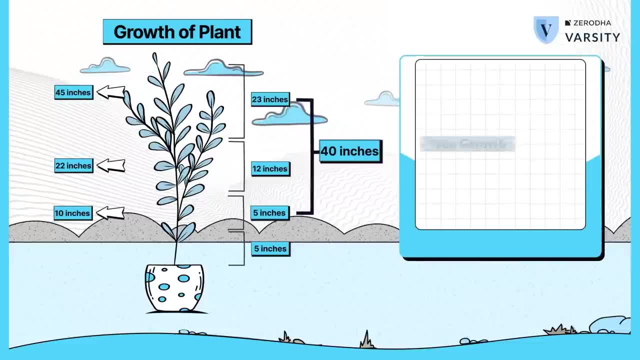 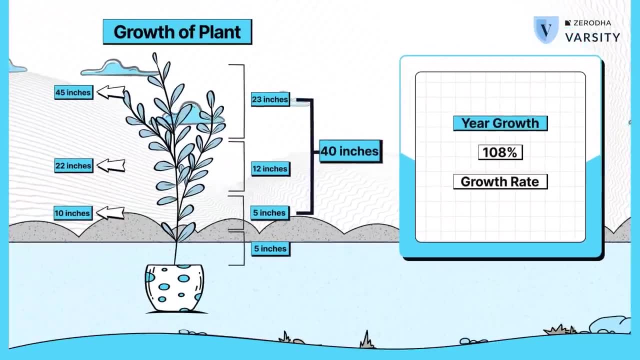 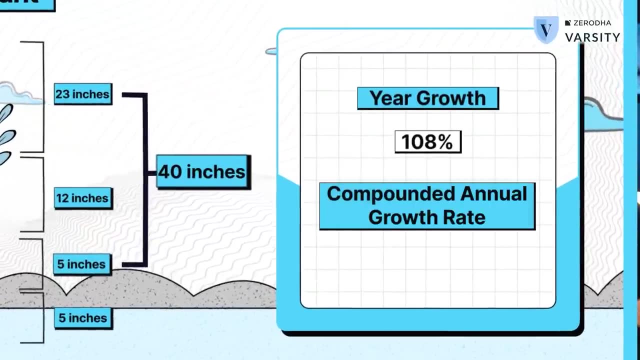 40 inches over 3 years, but the rate at which it has grown is 108%. Higher the growth rate, the better it is, especially for your investments. The formula that I used here to calculate 108% is also called the CAGR formula. CAGR, like I mentioned earlier, is the growth rate And the formula for CAGR is fairly straightforward and here is how it looks. Ignore the CAGR formula if it looks too complex for you, because most mutual funds publish the CAGR value anyway. However, it is super important that you understand what CAGR is and how to interpret the same. 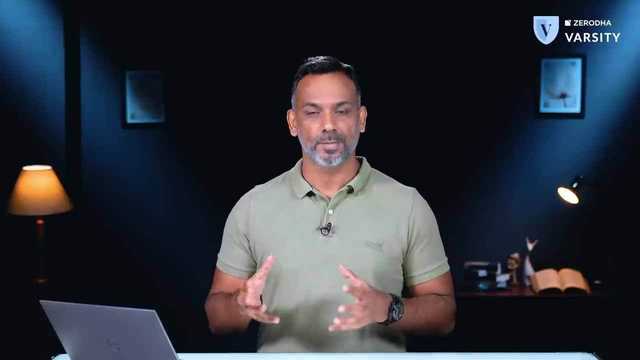 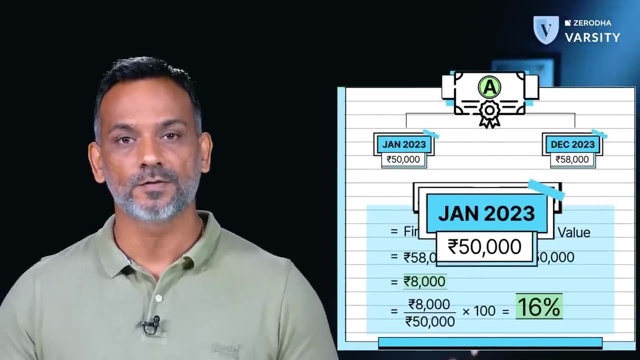 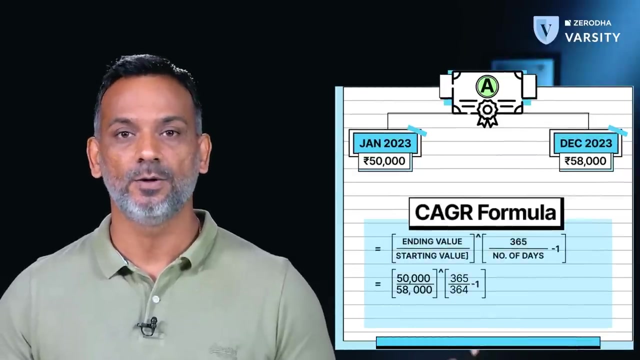 Now let's go back to our initial question as to which stock is better, stock A or stock B. The starting value of stock A is 50k, the ending value of stock A is 58k, and if you plug the CAGR formula here, you will get the CAGR value as. 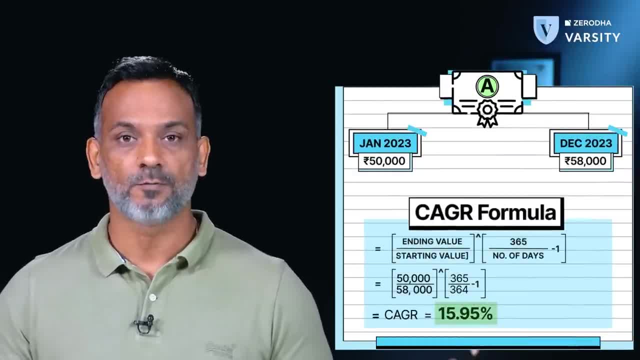 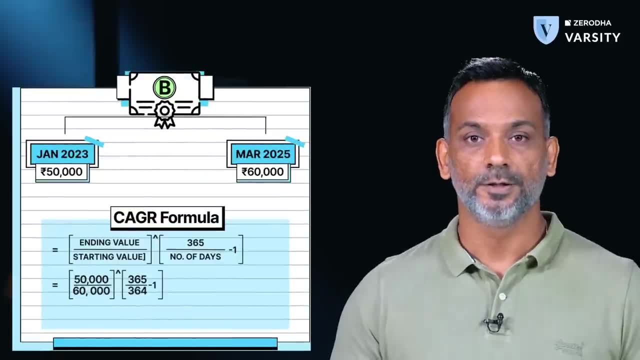 15.95%. Now if you do the same thing for stock B with the starting value as 50k and ending value as 60k and plug in the CAGR formula, you get the CAGR as 8.78%. So now you can compare both stock. 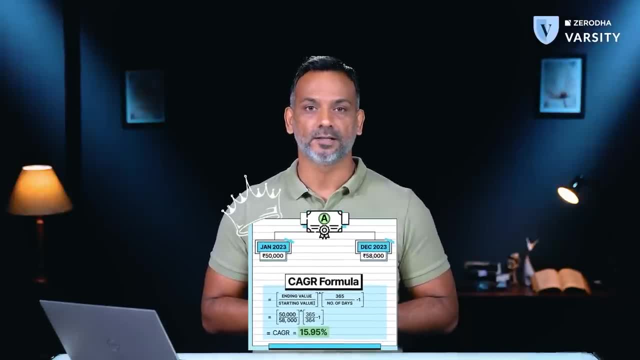 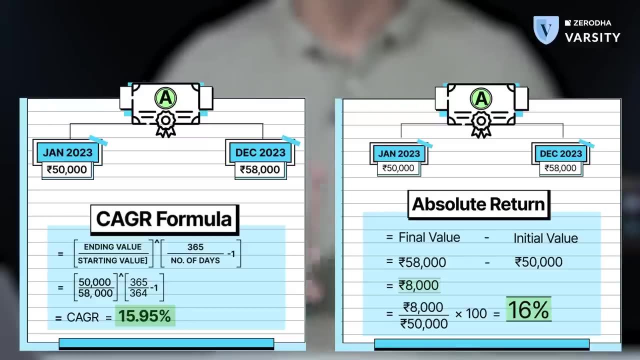 A and stock B and clearly stock A is the winner here. Let's stick to stock A for a bit. If you notice, the absolute return and the CAGR for stock A is nearly the same, that is 16%. Let's stick to. 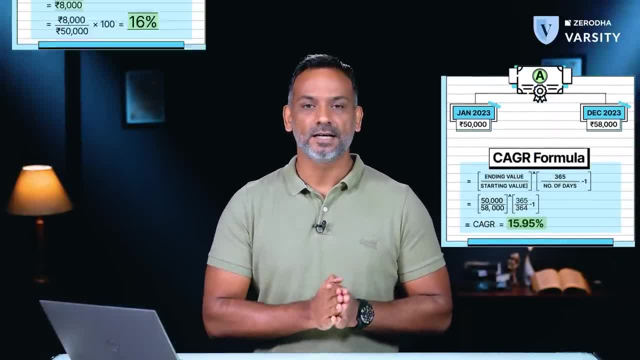 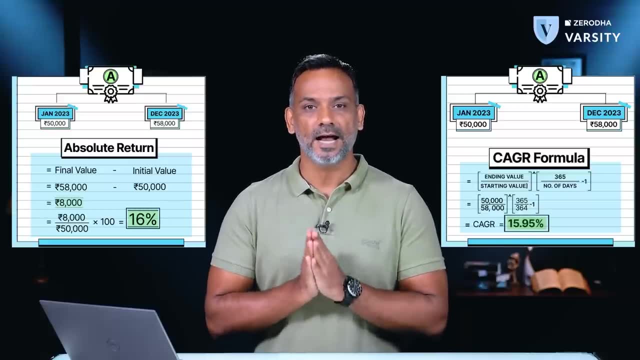 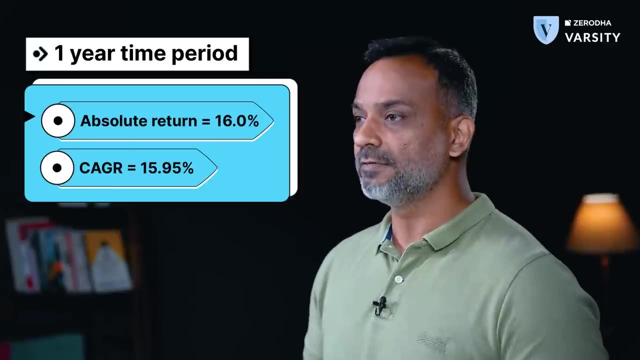 stock A for a bit. If you notice, both the CAGR and the absolute return is nearly the same, that is, 16%. Now, this is because both CAGR and absolute return will be the same as long as the time under consideration is exactly one year. But if the time is more than one year, then it's. 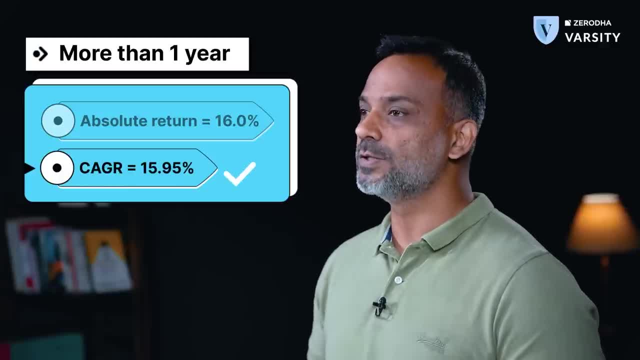 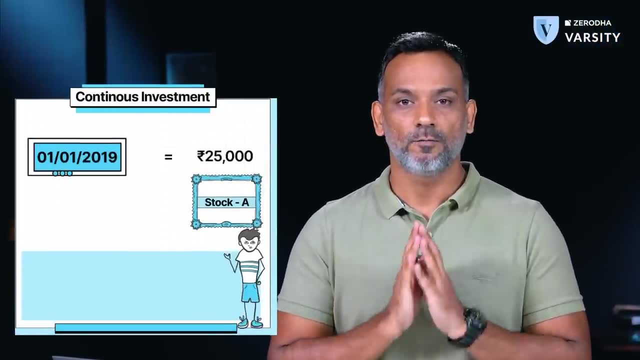 always better to look at the CAGR value as opposed to the absolute return. Now let's take another example. Assume that you make an investment of 25,000.. Assume that you make an investment of 25,000 on 1st of January for the next three consecutive years. That's basically 25,000. 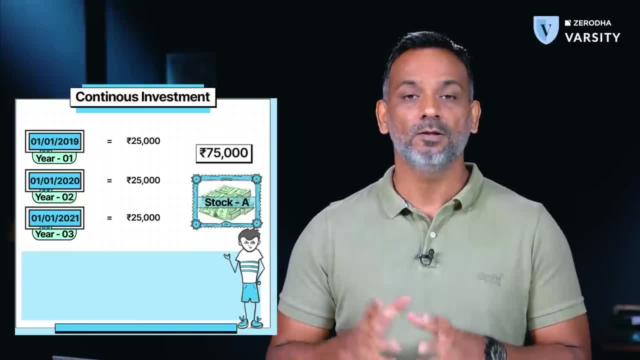 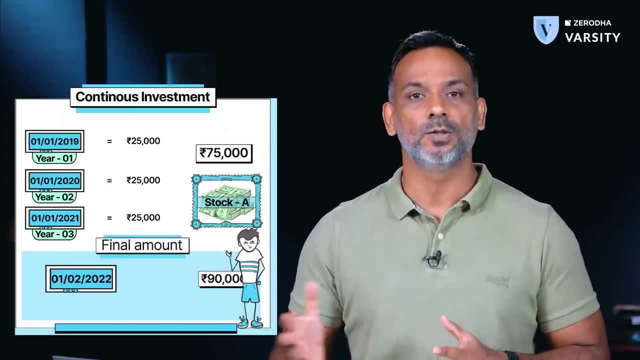 into 3, totaling up to 75,000. And on the 1st February of the fourth year you decide to withdraw all the money. Let's assume 75,000 has grown to 90,000.. What do you think is the return? 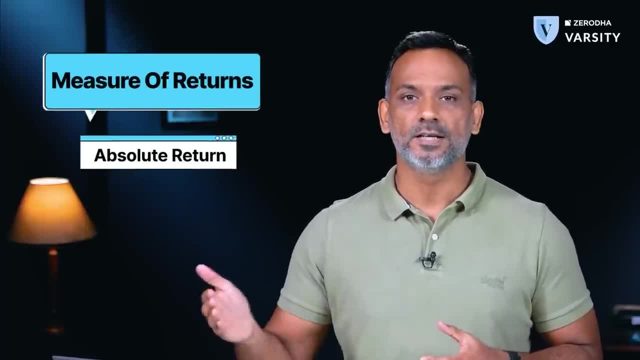 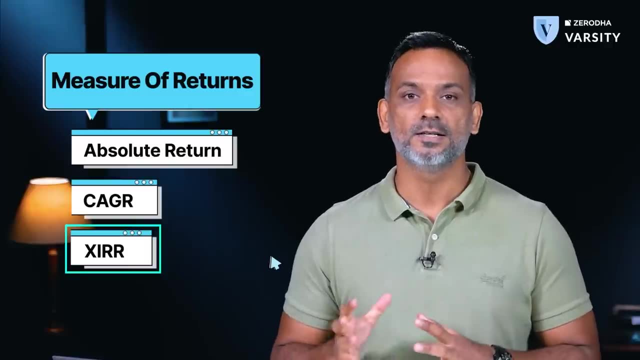 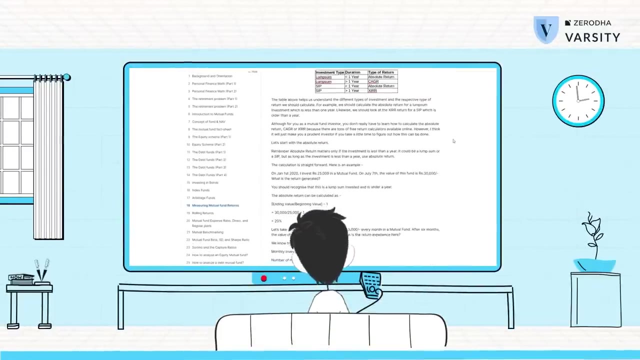 here. When you have to calculate returns for continuous investments, then you will have to calculate something called as XIRR. Think of XIRR as a close cousin of CAGR. I have discussed XIRR with examples in Varsity. I would suggest you give it a quick read. 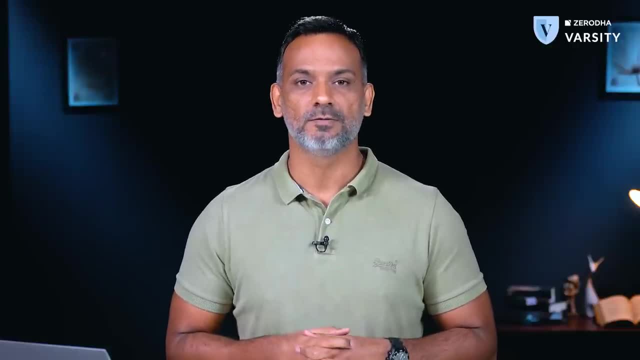 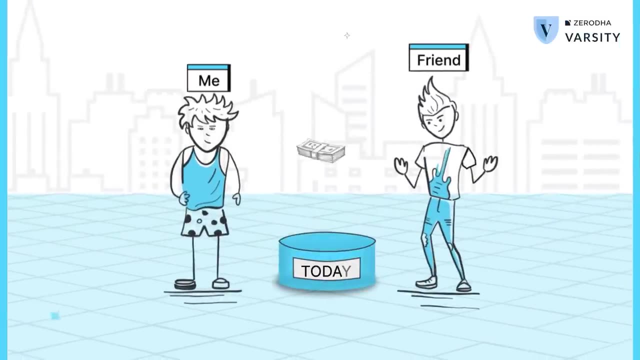 And with that we will now move to the next important concept in personal finance, That's the time value of money. Consider this: In return of a favour that you've done, your friend offers to pay you 84,000 today, or about 1 lakh in two years. 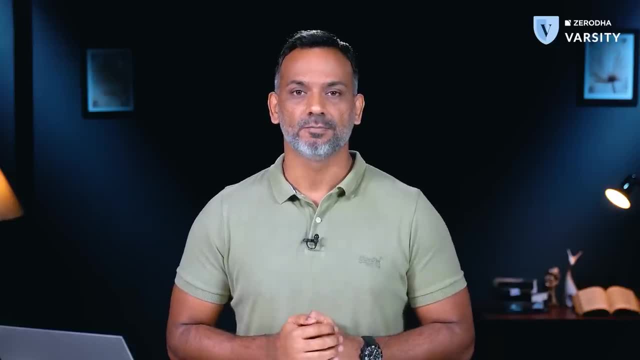 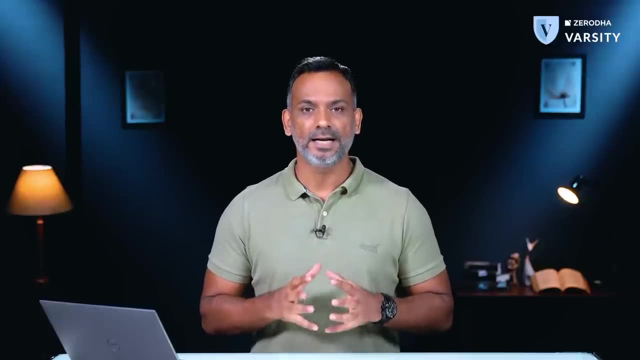 Which option will you take? This is a tricky situation. It's less money today versus more money in two years from now. Selecting an option blindly based on the magnitude of money can be a disaster, especially when you're comparing money across two different. 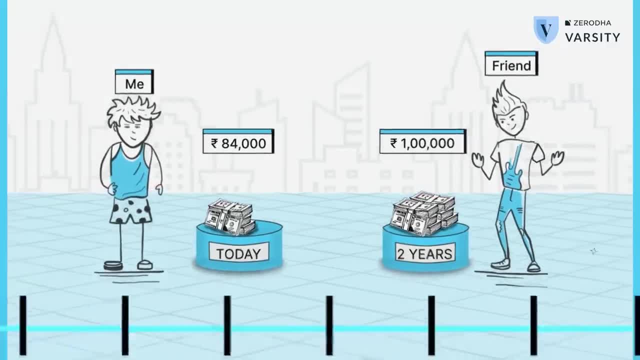 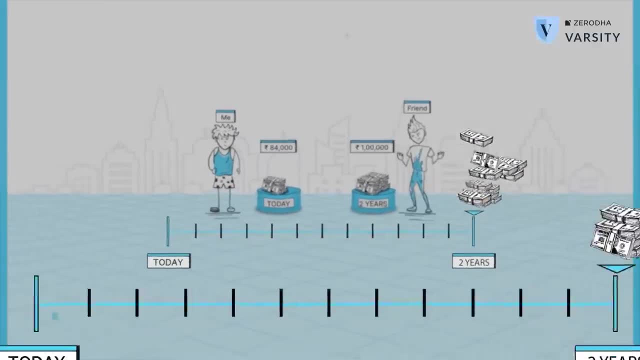 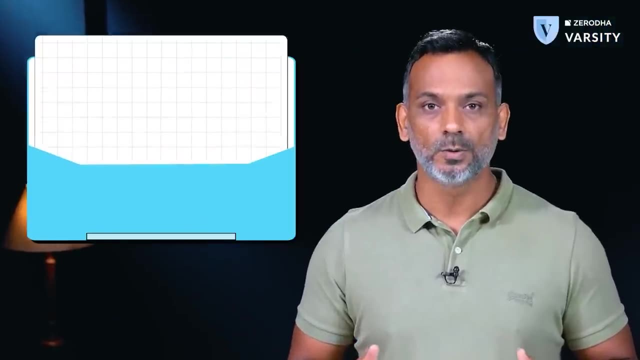 timelines To figure which is a better option. you will have to move 84,000 today to two years from now, or you'll have to bring 1 lakh back into today's value. Let's start with moving 84,000 two years forward. What we are about to do is called the future value of money. 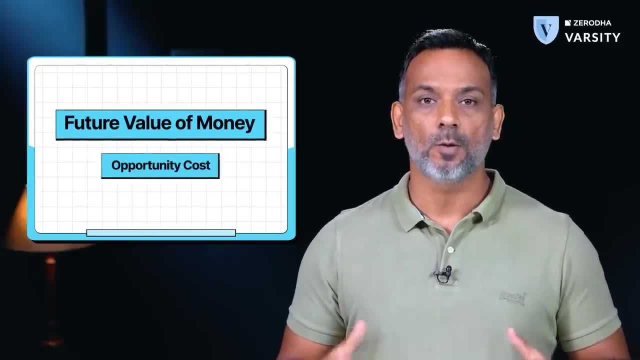 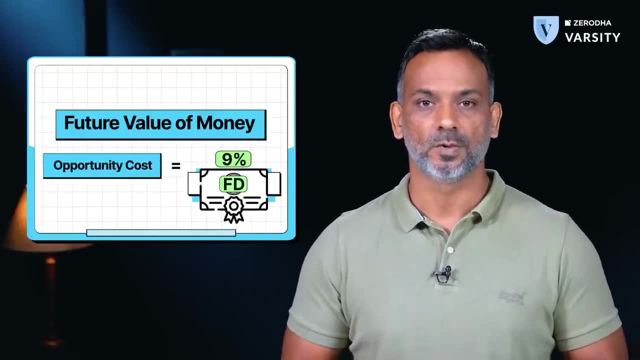 To do this, you need to first consider something called as the opportunity cost. Let's assume your friendly neighbourhood bank offers you a rate of 9% on a fixed deposit. For sake of simplicity, let's assume fixed deposit is a safe instrument. 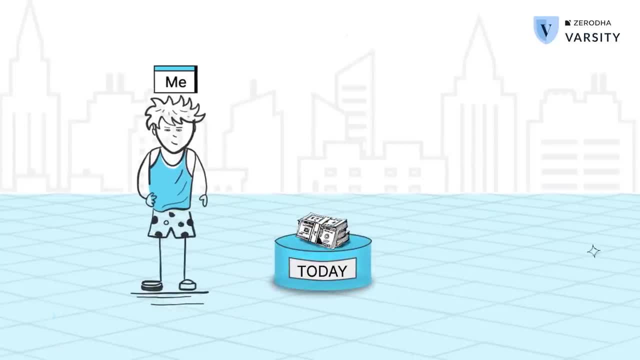 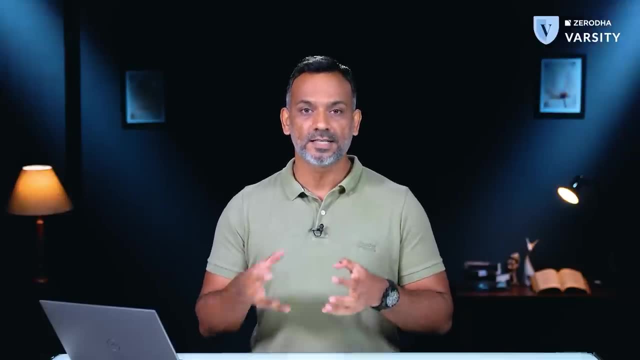 So if you were to receive 84,000 today, you can invest that in this opportunity, Basically the fixed deposit offering you 9%. So if you were to receive this 84,000 today from your friend and invest that in the opportunity, 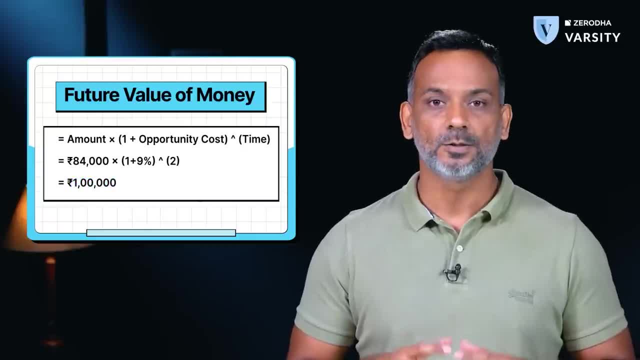 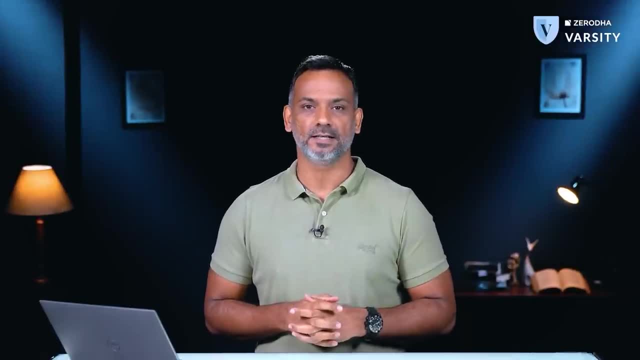 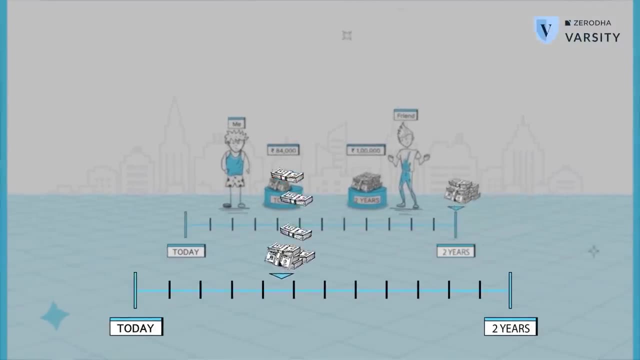 then in 2 years you will get 1 lakh. The math to do this is fairly straightforward, as you can see below Note: I have approximated the numbers here for easier understanding. Now let's try to bring 1 lakh 2 years from now into today's value. 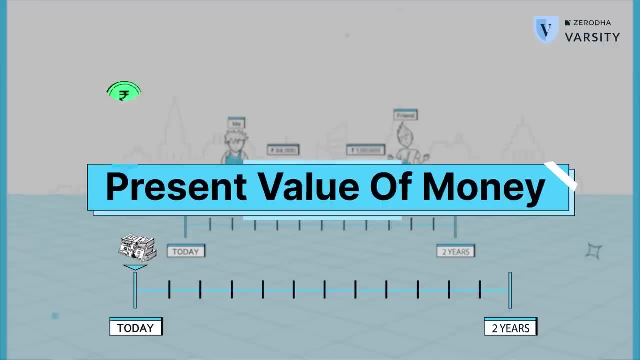 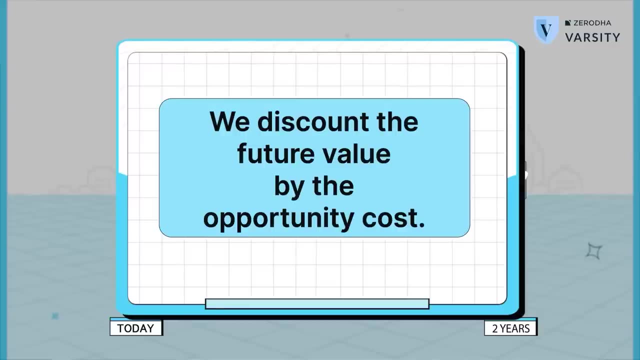 Bringing back the future value into today's value is called the present value of money. To calculate the present value, we need to discount the future value by the opportunity cost. The formula to calculate the present value is fairly straightforward, as you can see below. 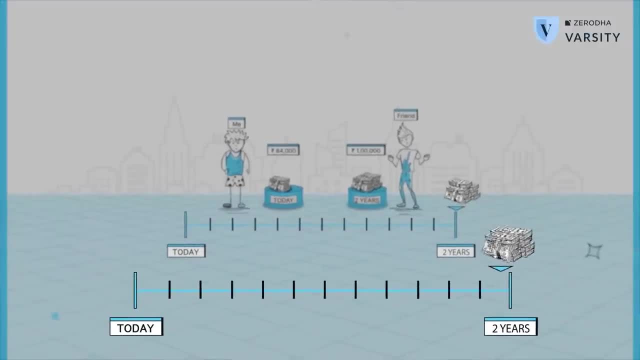 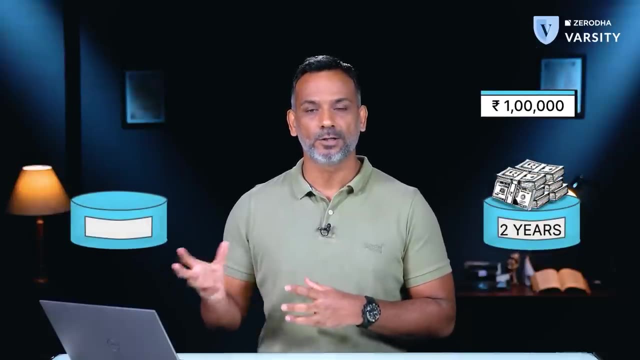 If you apply this math and bring back 1 lakh into today's value, by discounting it by the opportunity cost or the discount rate, you'll realize that 1 lakh in 2 years from now is as good as 84,000 today. 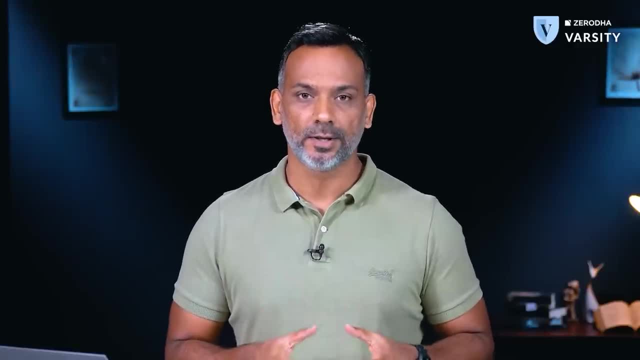 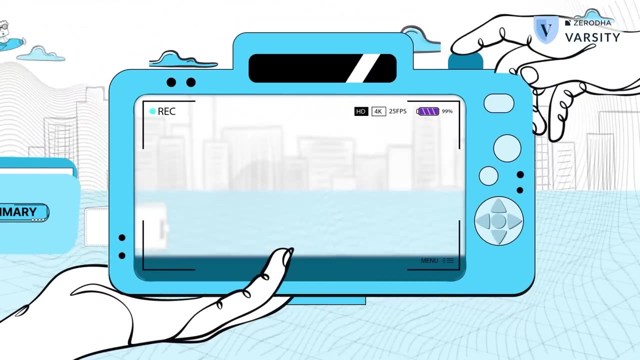 So the offer that the friend made, that is basically 84,000 today or 1 lakh in 2 years from now, is essentially the same and makes no difference. Let me wrap this video with a quick summary of all the things that we've learnt. 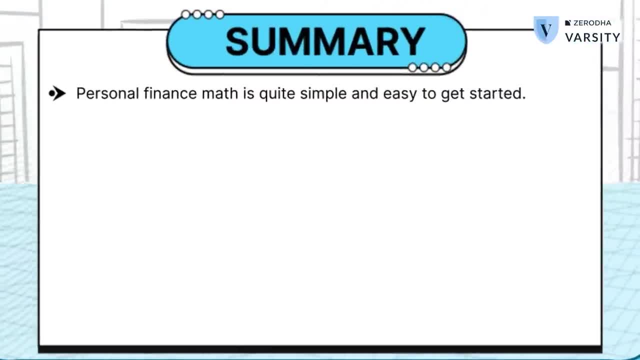 Personal finance is quite simple and you only need to know a handful of things to get started. Absolute return is used when you are calculating returns for 1 year. CAGR is a growth rate and is used when you are trying to calculate returns for more than. 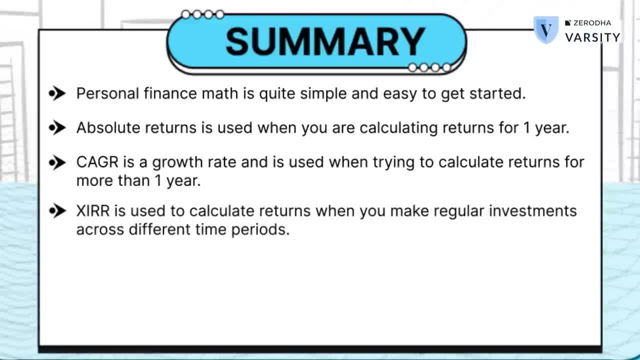 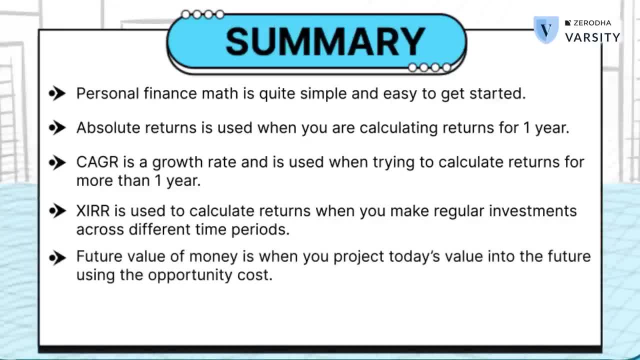 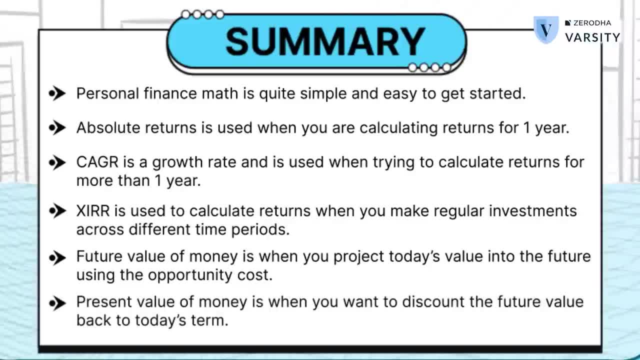 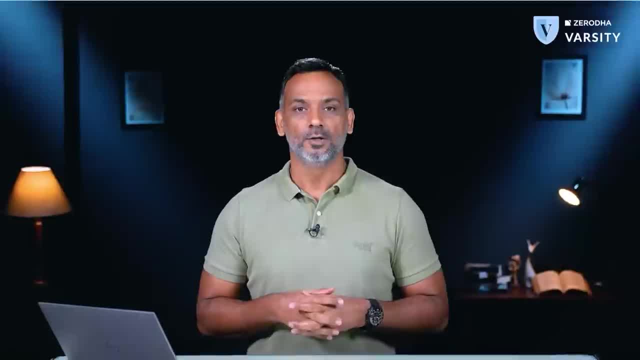 Current value of money is when you want to discount the future value into today's terms. With this in place, I guess you are now set to understand mutual funds better. Do comment and let me know if you have any queries with respect to all the. 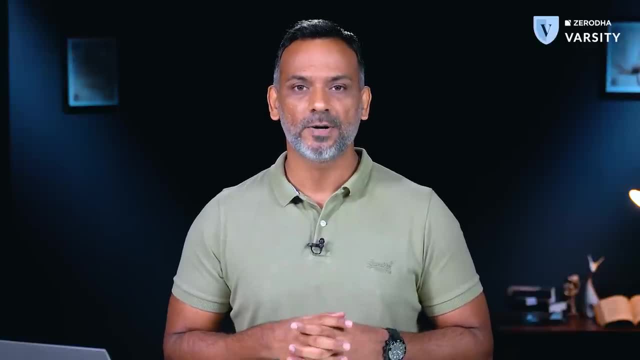 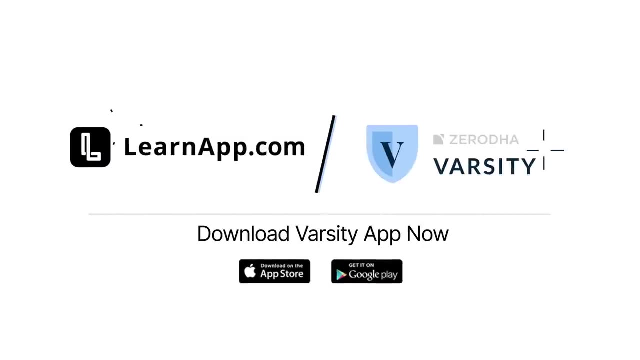 math that we've learned, and in the next video we'll dig a little deeper about mutual funds and understand the structure of an asset management company. Stay tuned, Thank you.